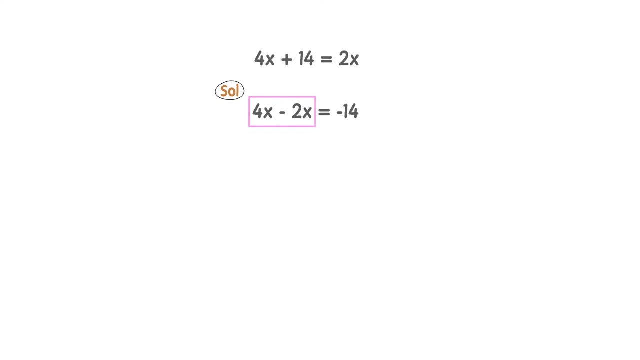 Now 4x minus 2x is equal to 2x. I get 2x is equal to negative 14. 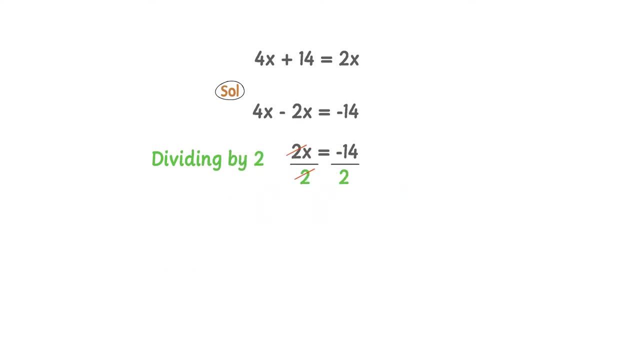 Dividing both sides by 2, this 2 and this 2 are cancelled out. Minus 14 upon 2 is equal to negative 7. So, I get x is equal to negative 7. This is the solution set of this linear equation. Now let me take you to the medium level. 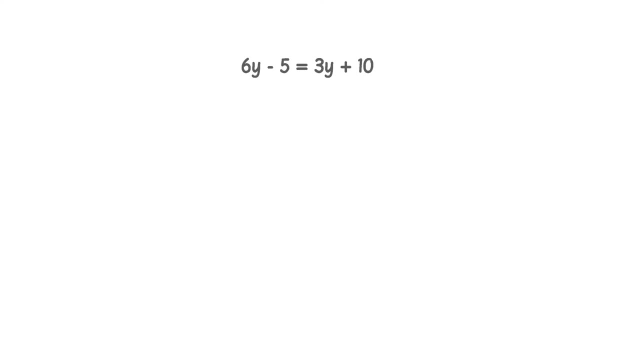 Consider 6y minus 5 is equal to 3y plus 10. 6y and 3y are variable terms while negative 5 and positive 10 are constant terms. 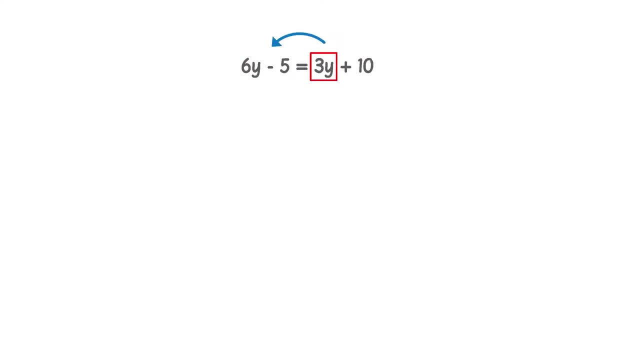 So, I shift the 3y from the right-hand side to the left-hand side and I shift negative 5 from the left-hand side to the right-hand side. 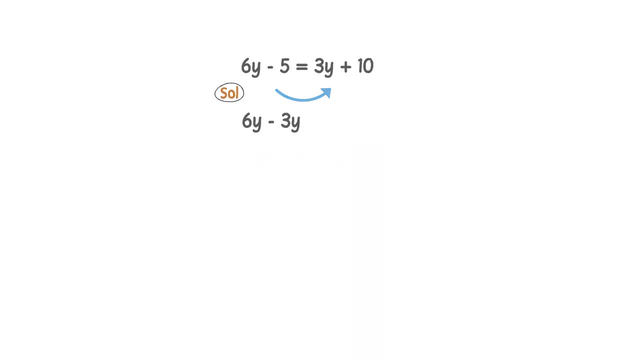 I get 6y minus 3y because the positive sign of 3y changed is equal to 10 plus 5 because negative sign of minus 5 changed. Now 6y minus 3y is equal to 3y and 10 plus 5 is equal to 15. 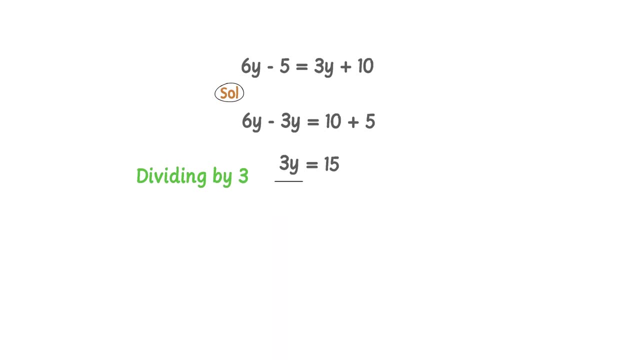 Or 3y is equal to 15. Now dividing both sides by 3, I get y is equal to 5. This is the solution set of this linear equation. 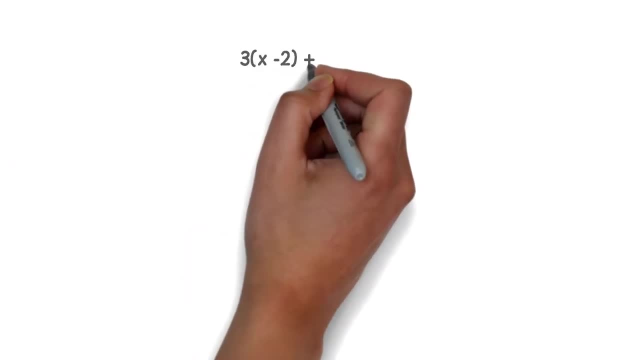 Consider one another linear equation. 3 into x minus 2 plus 4 is equal to 2x. And such type of linear equations always solve the bracket to get simple linear equation. 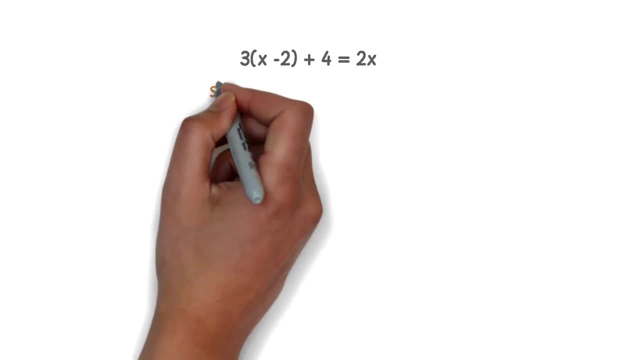 For example, 3 into x is equal to 3x and 3 into negative 2 is equal to 3x. 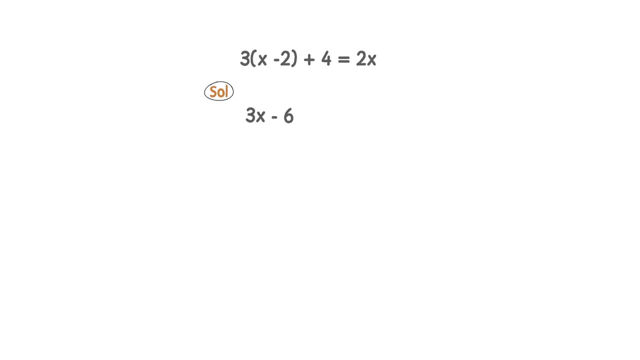 Bring down the remaining parts as positive 4 is equal to 2x. 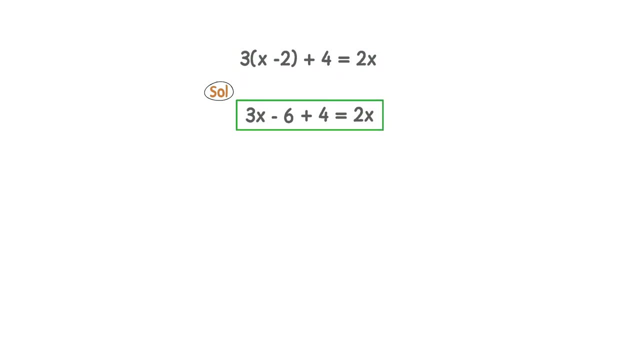 Thus, I simplified this linear equation to this linear equation by dissolving the bracket part. 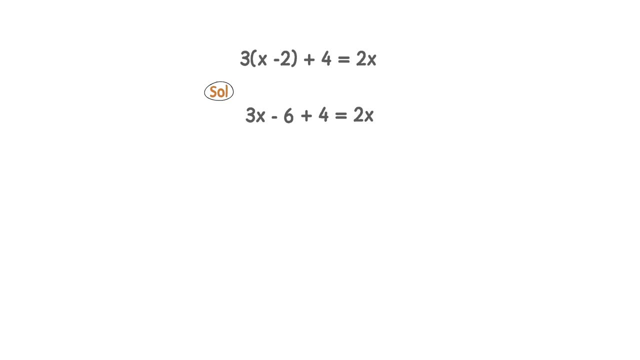 Now I will separate variable terms and constant terms. I shift 2x to the left-hand side and I shift negative 6 positive 4 to the right-hand side. I get 3x minus 2x is equal to 6x. 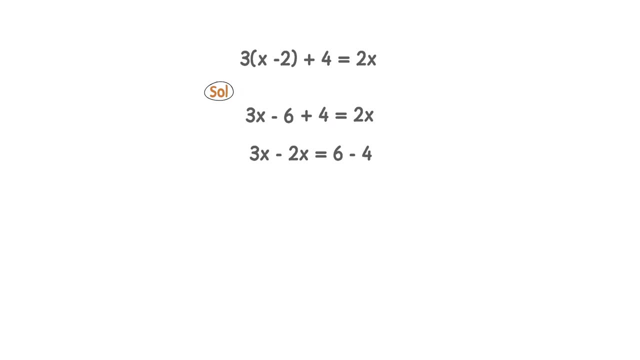 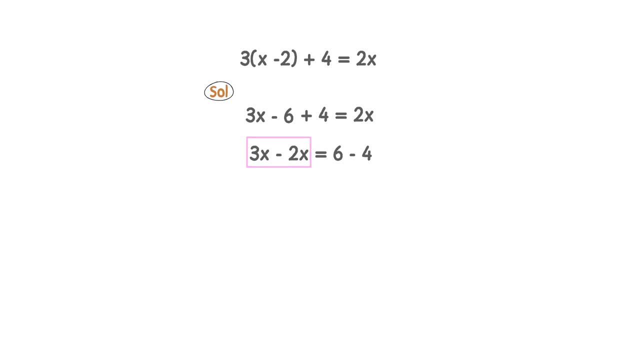 Now, 3x minus 2x is equal to x and 6 minus 4 is equal to 2. Thus, I get x is equal to 2. 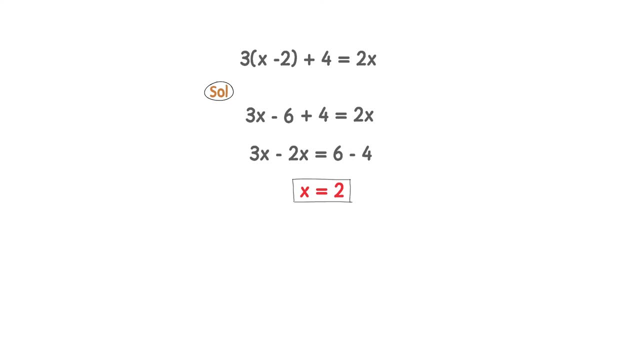 This is the solution of this linear equation. 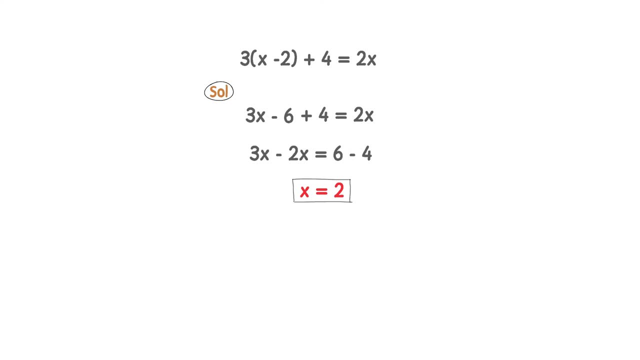 Finally, let me teach you difficult linear equation. For example, 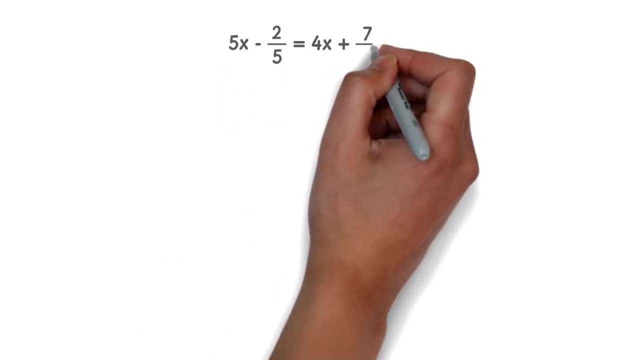 5x minus 2 upon 5 is equal to 4x plus 7 upon 2. Now, I will separate the variable terms and constant terms 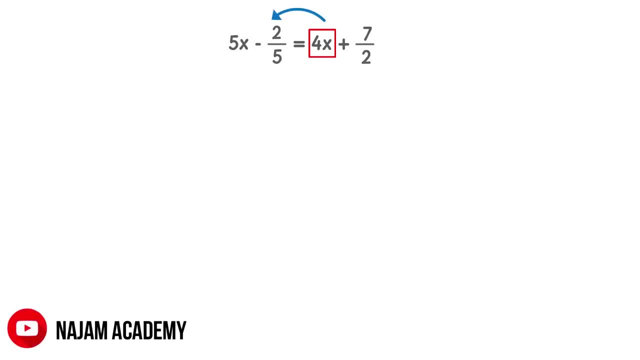 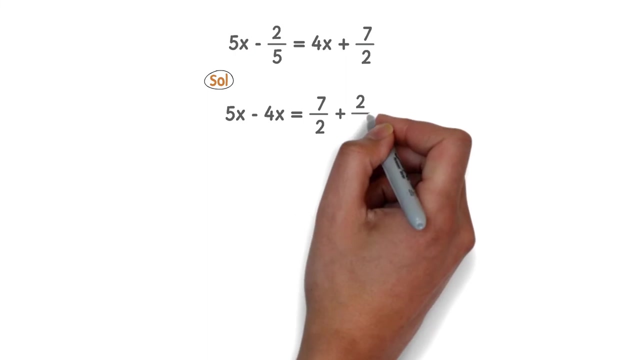 constant terms. I shift 4x from the right-hand side and I shift minus 2 upon 5 from the left-hand side and their signs change. Hence, I get 5x minus 4x is equal to 7 upon 2 plus 2 upon 5. Now, 5x minus 4x is equal to x. Bring down the remaining part is equal to 7 upon 2 plus 2 upon 5. Now, I will take the LCM of 2 and 5 and we know that its LCM is 10. I need to multiply this 2 with such a number and denumerator so that I get 10. I know it is 5. So, I also multiply it in the numerator. Again, I need a number to be multiplied with this 5 and denumerator so that I get 10 and I know it is 2. So, I also multiply it. In the numerator, I get x is equal to 7 and 5 is equal to 35 upon 2 and 5 is equal to 10 plus 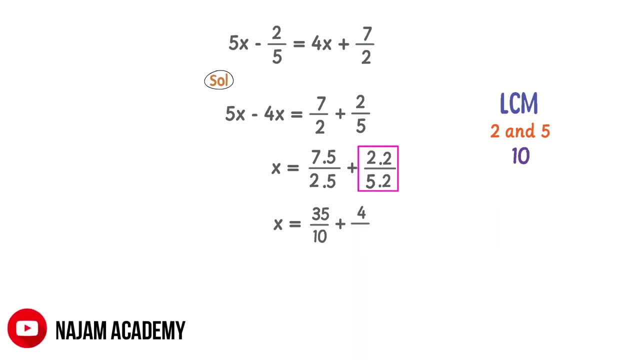 2 and 2 is equal to 4 upon 5 and 2 is equal to 10 or x is equal to 35 plus 4 upon 10. Thus, I get x is equal to 39 upon 10. This is the solution of this linear equation. 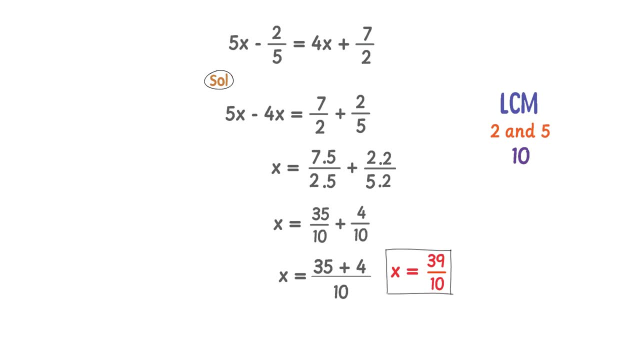 Therefore, by this way, we can solve any linear equation easily. I hope that you have learned this method of solving linear equation.